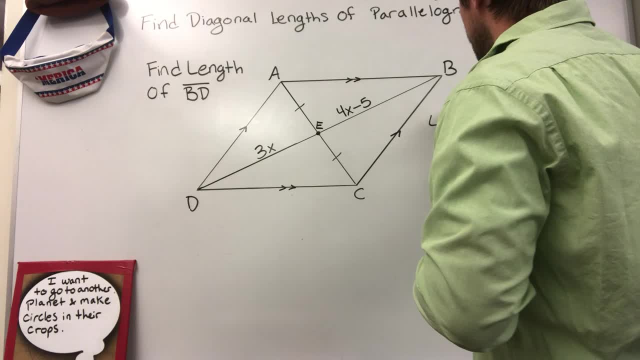 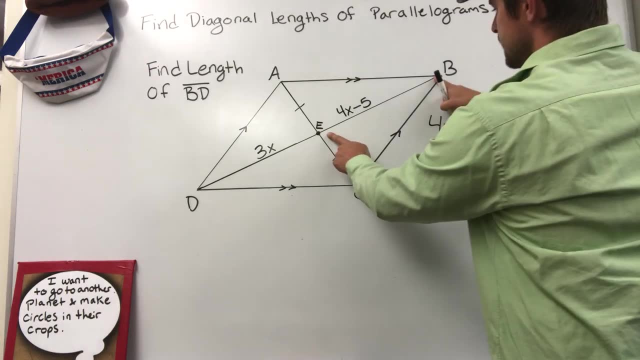 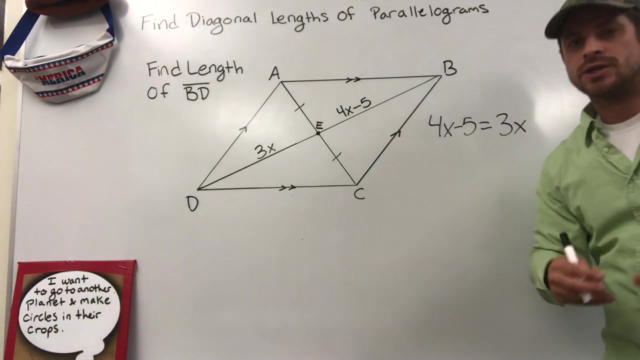 We know they're equal, so I'm going to write an equation that represents that 4x minus 5 equals 3x. This is essentially the same length as this, So I write an equation that represents that. Now I solve that equation just like you did in your Algebra 1 classes. We need to solve for x. 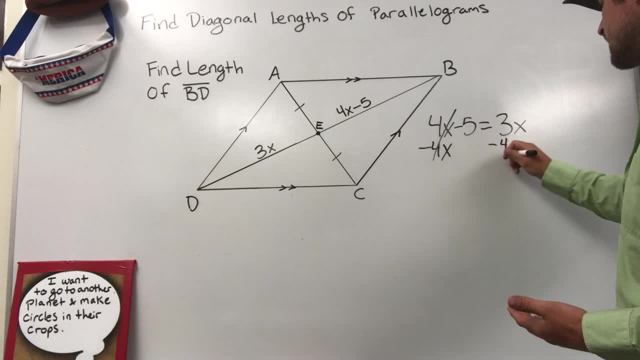 so we're going to take away 4x. Cancels. take away 4x, That's going to leave us with negative 1x equals negative 5 divided by negative 1.. Cancels divide by negative 1.. And that gives me x equals a. 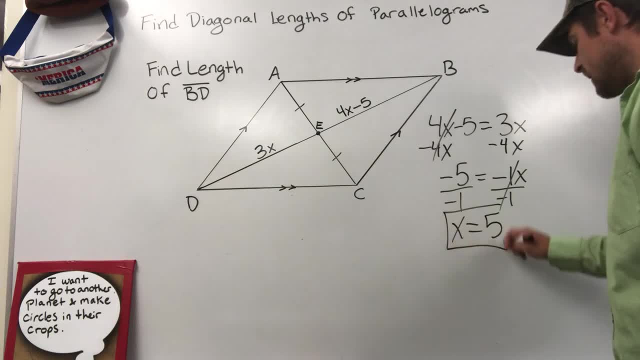 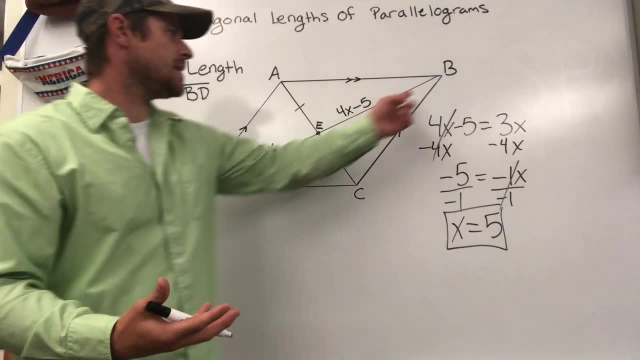 negative divided by a negative is a positive. So right now I know x is 5. And students every single year in my class will say 5 is their answer. They'll say DB or BD line segment. BD is five inches five feet. 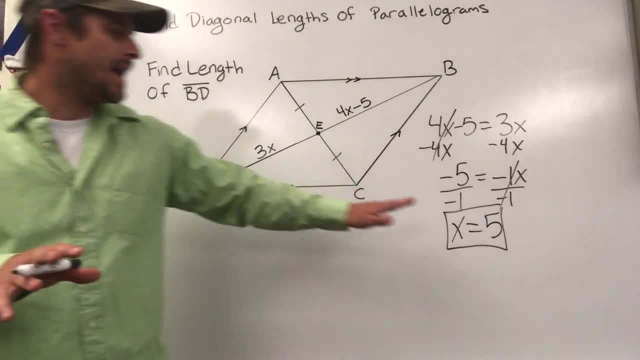 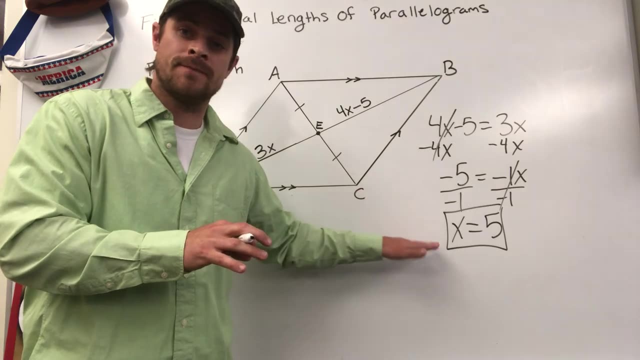 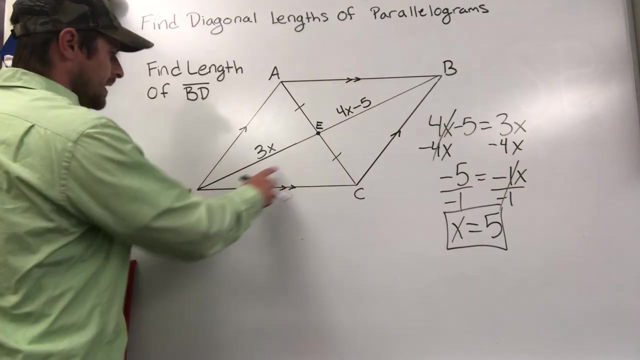 however many five long, But it's not. X is five. So the common error, the common mistake that I see in my class is students will say five is the length, but 5 is not the length. 5 is just representing the value of x. So what we need to do to figure out the length. 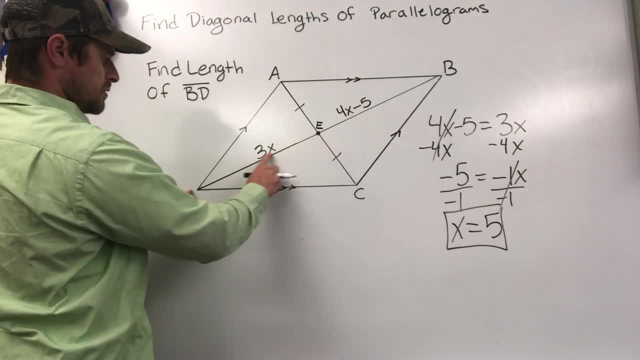 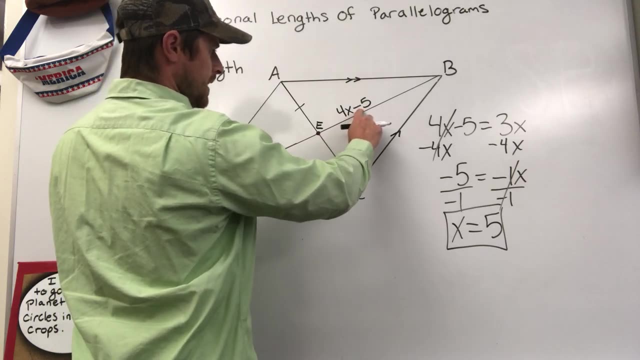 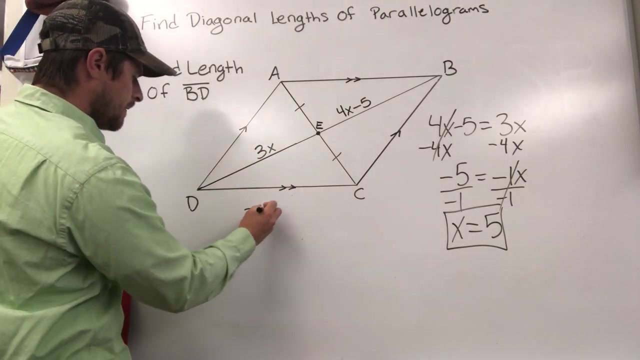 if you're asked to find DE, just say 5 times 3 or 3 times 5. if you're asked to find BE, 4 times 5 minus 5. remember X is 5, so we're just gonna plug that in. so let's plug it into this one, quick and easy. 3 times 5 gives me 15. therefore, D to 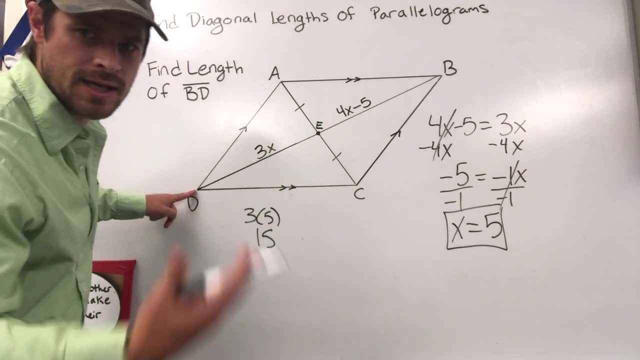 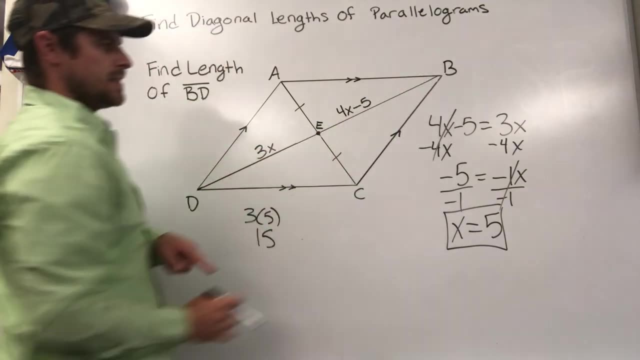 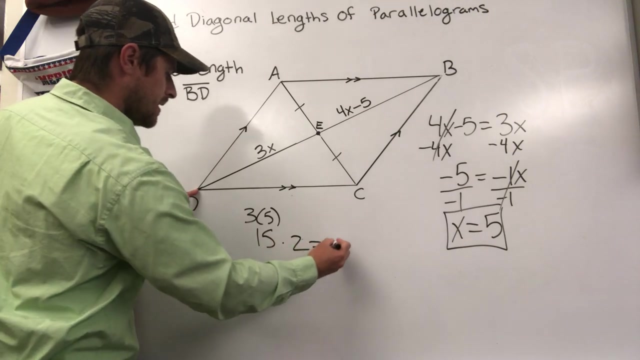 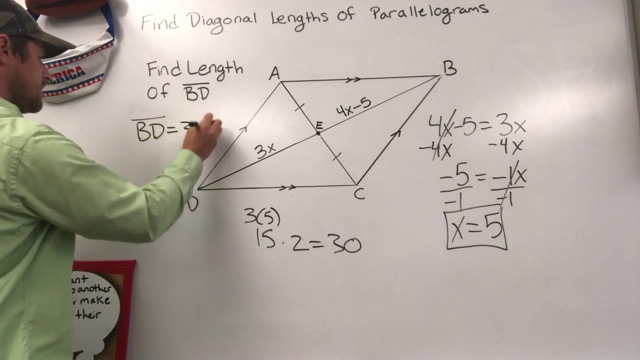 E is 15. let's say our unit of measure is inches, this would be 15 inches. if this is 15 inches, this is also 15 inches and they want to know what BD is all the way across. so two 15s make 30. our answer here is: line segment B D is 30, hopefully. 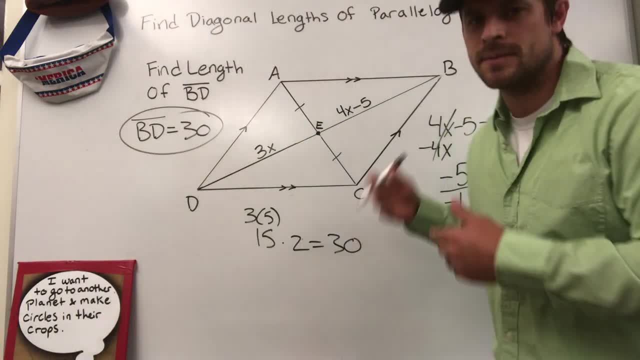 this makes sense. study hard and good luck on your upcoming tests. Parallelograms.